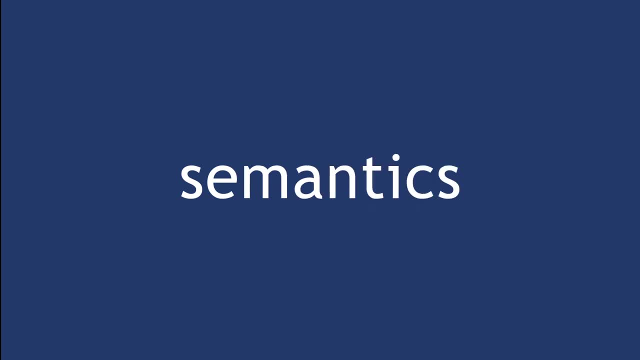 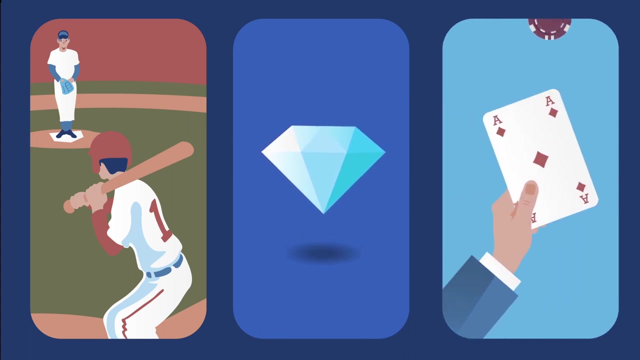 dissertation. This is part of a branch of linguistics called semantics, the study of meaning. For example, the word diamond can have a very different meaning depending on the context, such as when used by a baseball player, a jeweler or a poker player. Determining. 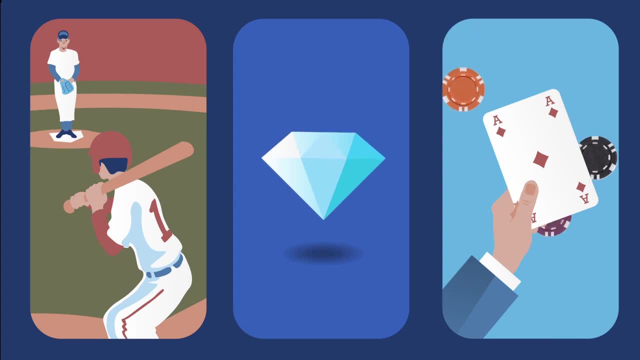 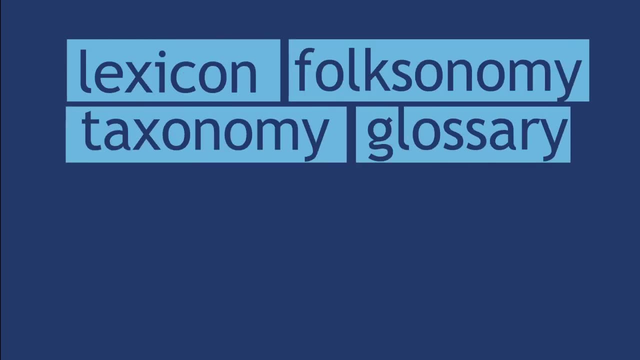 which one is applicable for a given situation can be difficult for humans, let alone computers, To explain what an ontology is. we begin by discussing these related linguistic terms. They all differ by their level of complexity, but what do all of these terms have in common? 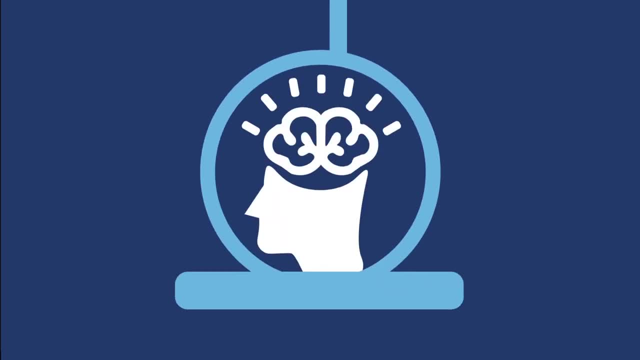 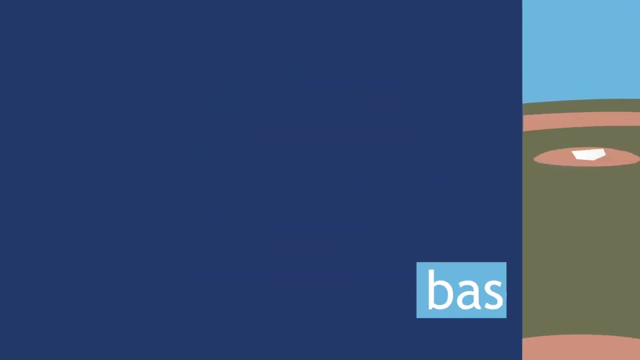 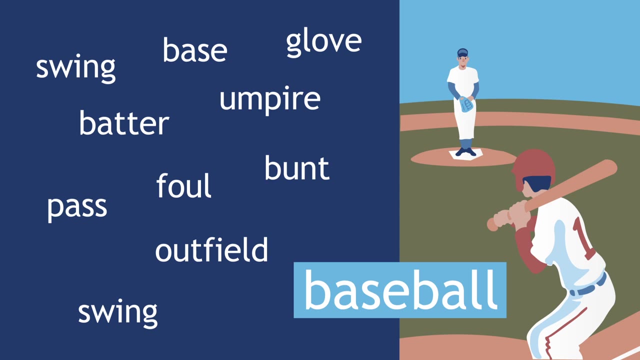 They all define a collection of terms that are associated with a set of related information or a knowledge domain. Let's visit each one, beginning with the least complex. A lexicon is just a collection of words, terms and phrases associated with a knowledge domain. 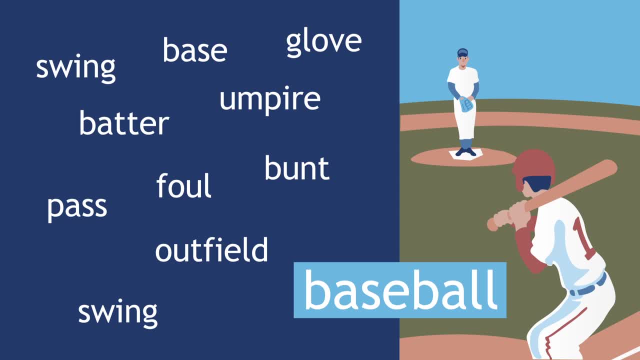 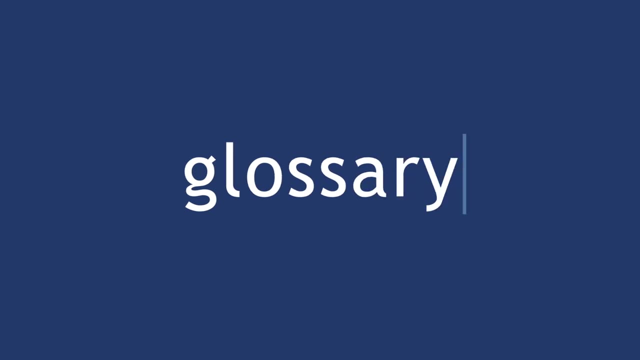 There is no other context provided in a lexicon: No definitions, no explanations of how terms are related, no prioritization of significance. A lexicon is roughly equivalent to a vocabulary. A glossary is like a lexicon, but with glosses added. A gloss is just a fancy linguistic. 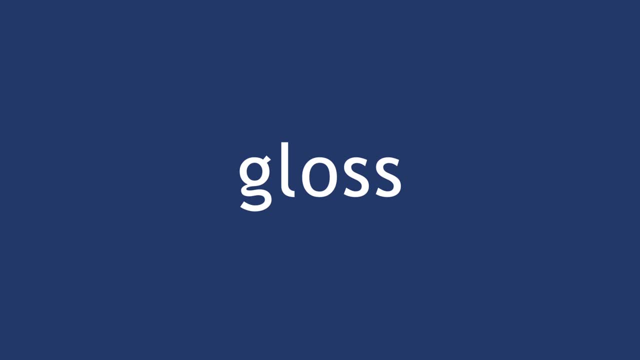 term for a definition. Usually, each term has only a single definition, provided the one that is applicable to the knowledge domain associated with the glossary. For example, the definition for diamond in a glossary of baseball would be, for example, the definition. 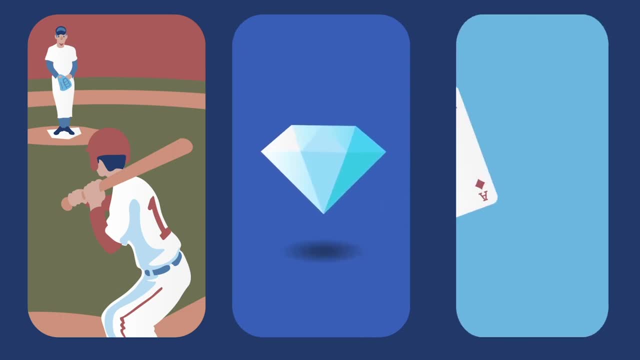 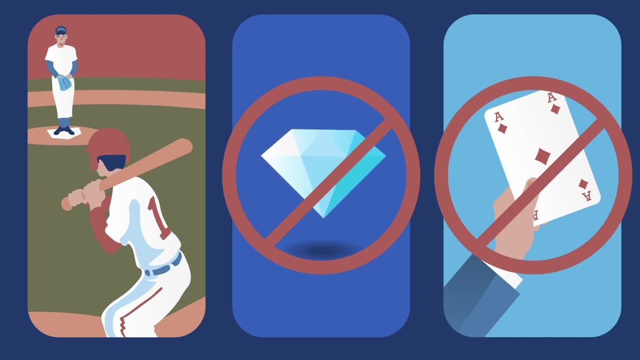 of diamond in a glossary of baseball. But in a glossary of baseball the definition of ball wouldn't mention anything about the context of the word in jewelry or poker. Even though there is no inherent order or structure to a glossary they usually list. 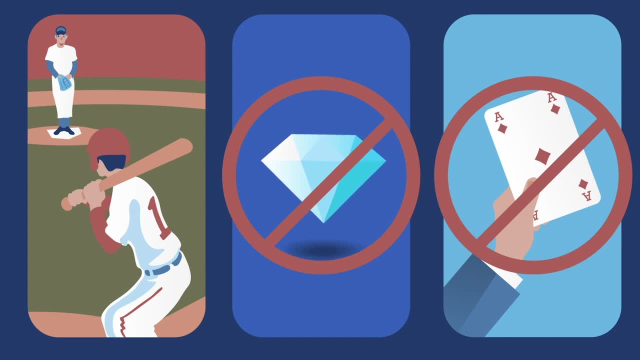 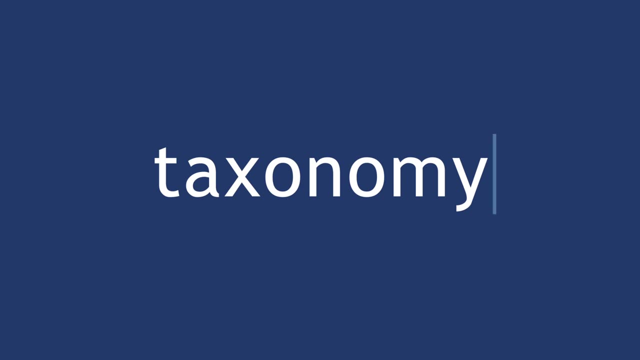 terms alphabetically to accommodate easier search and lookup by humans. A taxonomy usually lacks the definition of a glossary, but the terms are organized by their relationship to one another in the form of a hierarchical tree. Most of the time this relationship is by hypernomy, also called the is-a relationship. 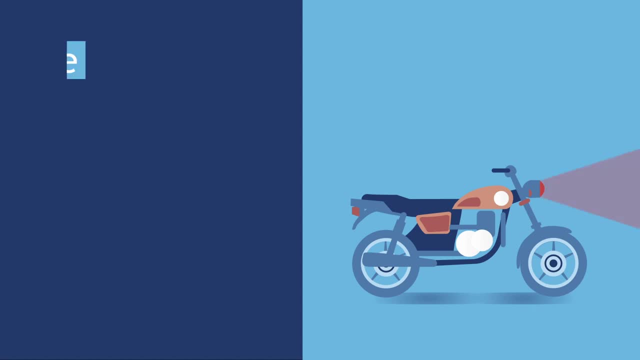 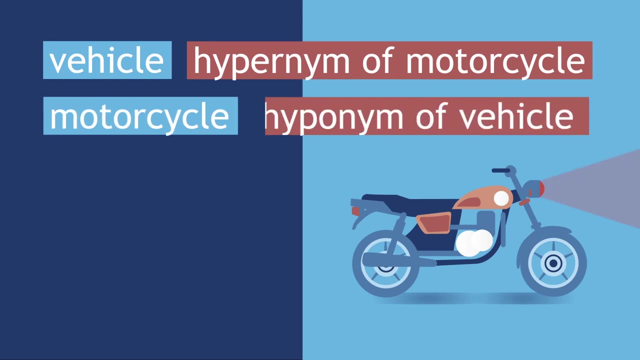 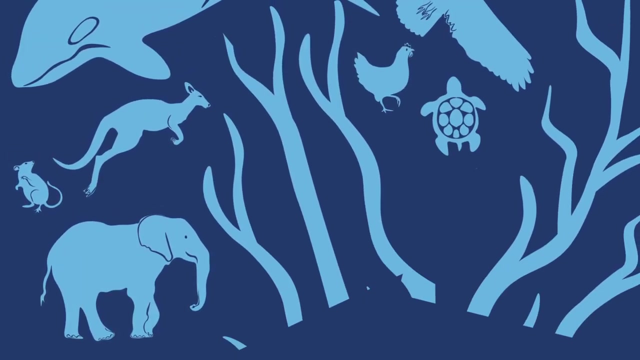 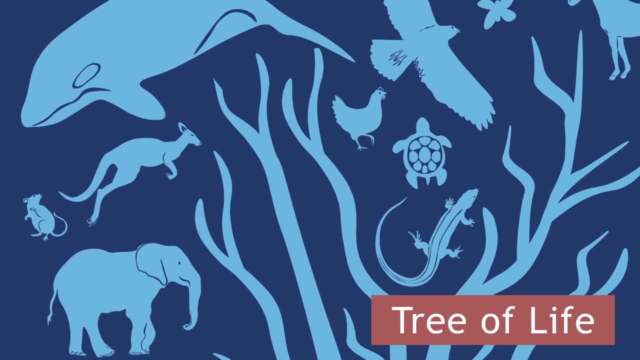 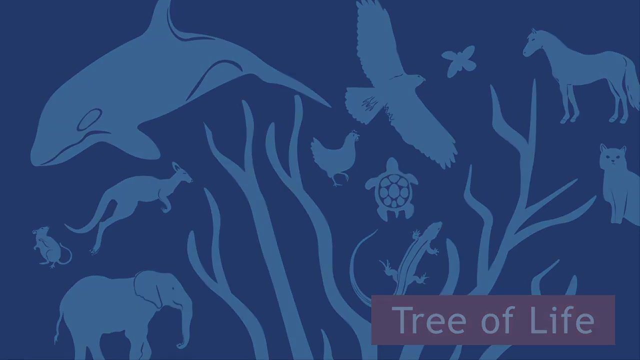 If motorcycle is a vehicle, then vehicle is a hypernym of motorcycle and motorcycle is a hyponym of vehicle. Many of us encountered our first wide-reaching taxonomy in middle school learning: the biological tree of life Organized by kingdom, phylum, class, order, family, genus and species. 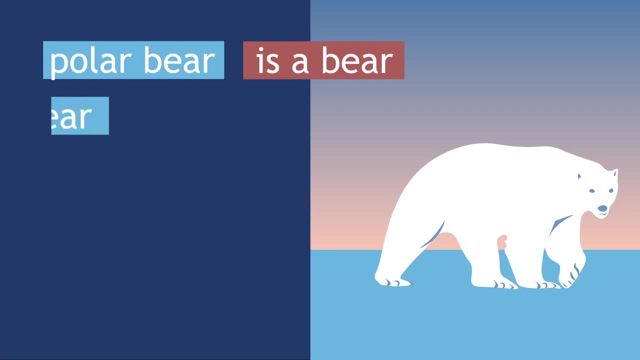 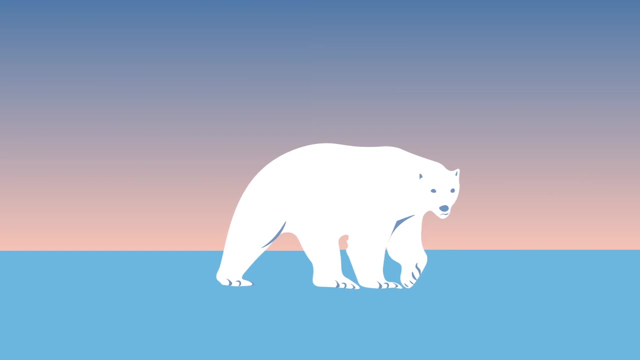 A polar bear is a bear, A bear is a mammal, A mammal is a vertebrate, and so on. Most of the time, attributes possessed by a concept higher in a taxonomy are also held by its sub-concepts. For example, an attribute of phylum Chordata is possessing a spinal cord. 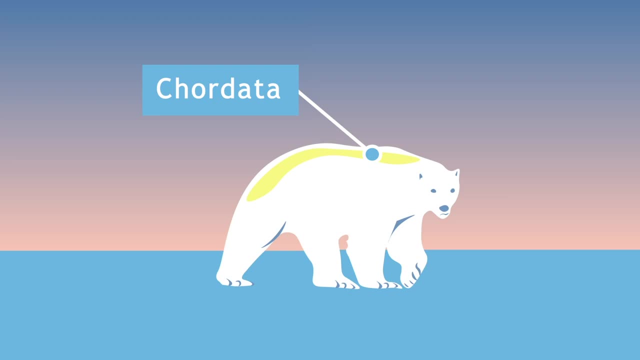 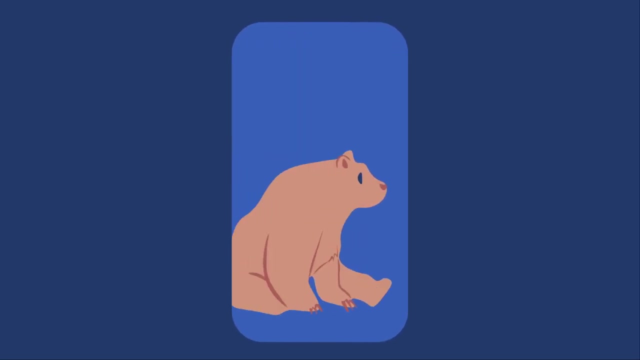 Therefore, as a subtree of phylum Chordata, bears have a spinal cord. The ability to classify concepts and then draw inferences based on category memberships allows for great predictive analytical power. The same concept of a bear as an animal may appear in different taxonomies that are organized. 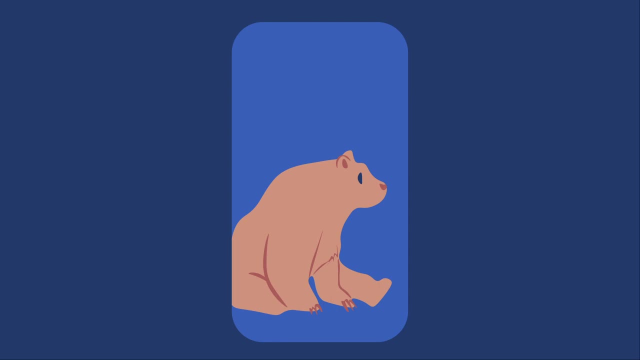 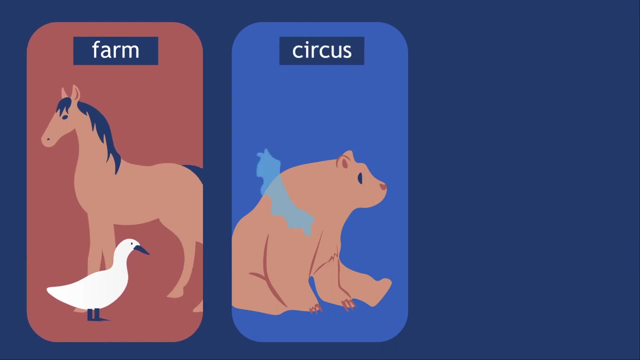 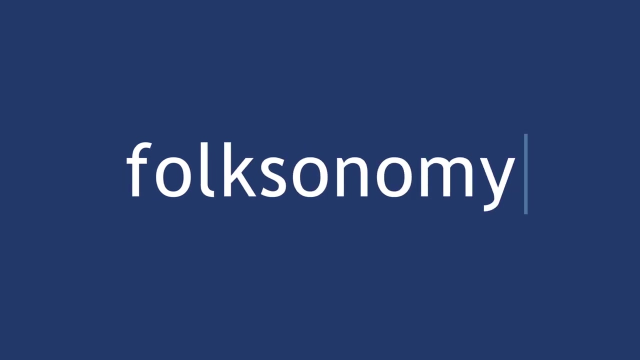 by different criteria. Perhaps another taxonomy classifies animals by geographic region or their association to humans, such as farm animals, circus animals or work animals. A folksonomy shares features of both a lexicon and a taxonomy, but not deeply structured as a taxonomy. 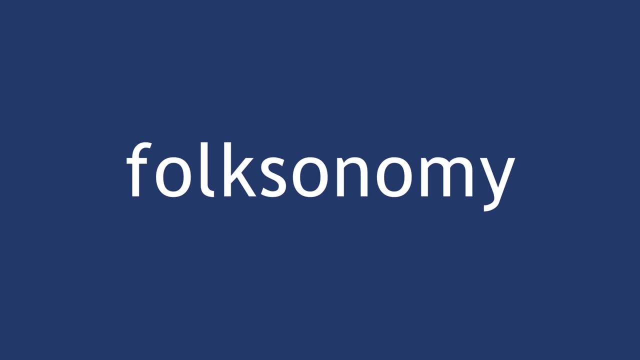 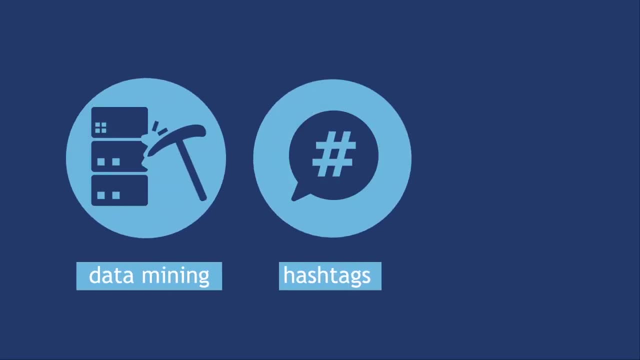 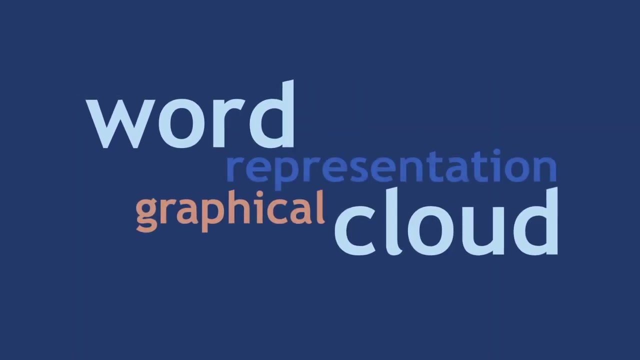 The primary identifier of a folksonomy is that it is created organically through crowdsourcing of metadata about a knowledge domain, usually by data mining, hashtags or word counts. One type of folksonomy is a word cloud, a graphical representation of the frequency. 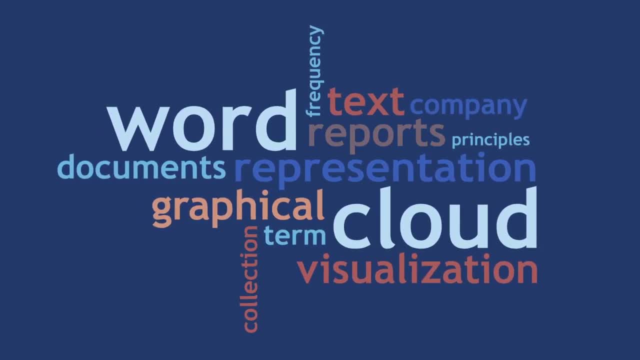 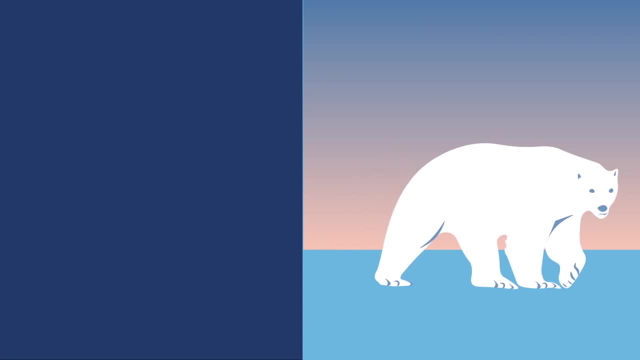 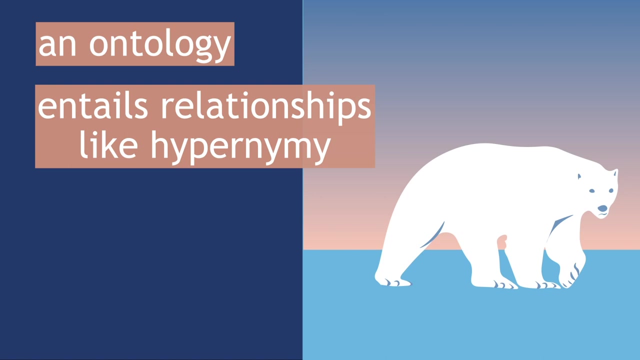 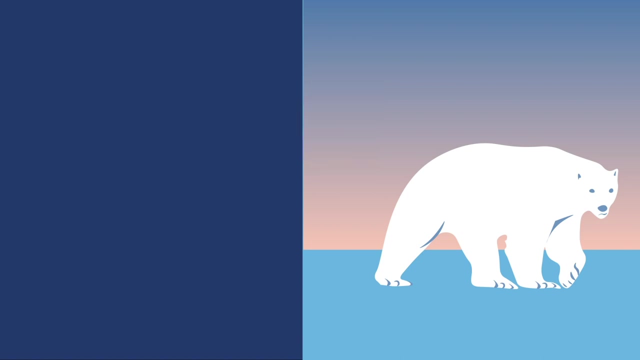 a term appears in some collection of text. The more frequent the term, the larger the term appears in the graphic Like a taxonomy. an ontology entails relationships like hypernomy. An ontology may have hypernomy relationships from multiple overlapping taxonomies.